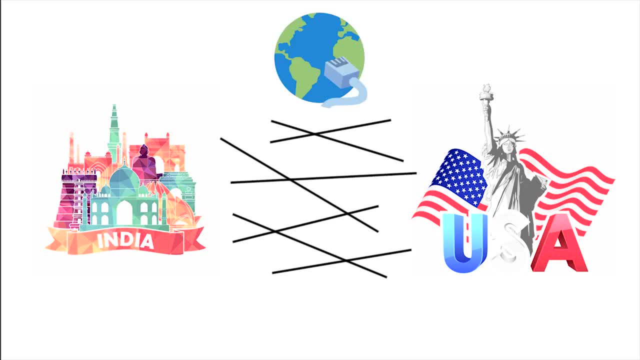 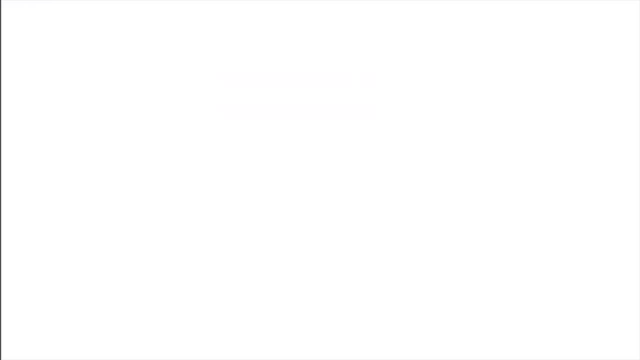 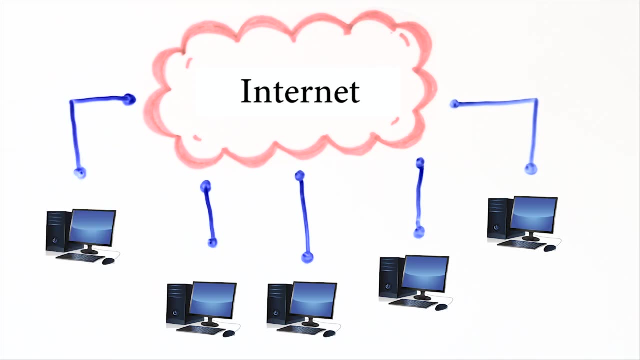 across cities, countries and continents. It is also known as Internet Savi. how big is this Internet? The Internet is the world's largest network. The Internet connects millions of computers to one another. These computers can share information with each other. 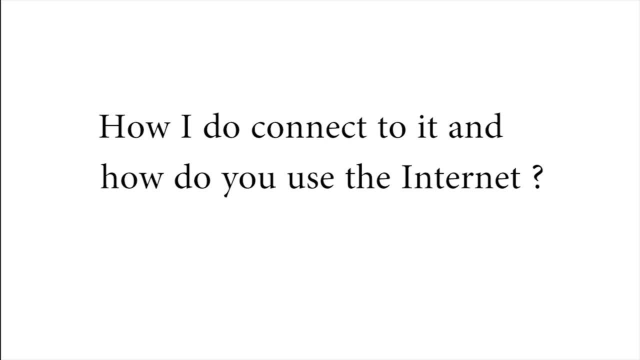 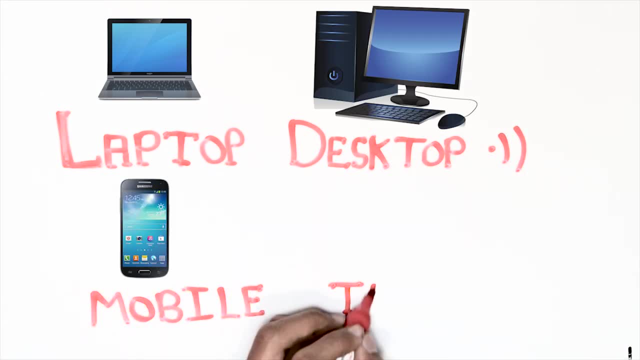 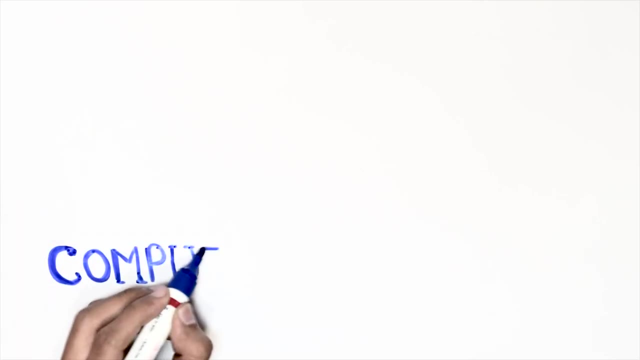 How can I connect to it And how do you use the Internet? You can connect to Internet on your laptop, desktop tablets, mobiles, etc. You can connect using cables or wireless mediums. First, a computer is connected to a modem using cables or wireless mediums. 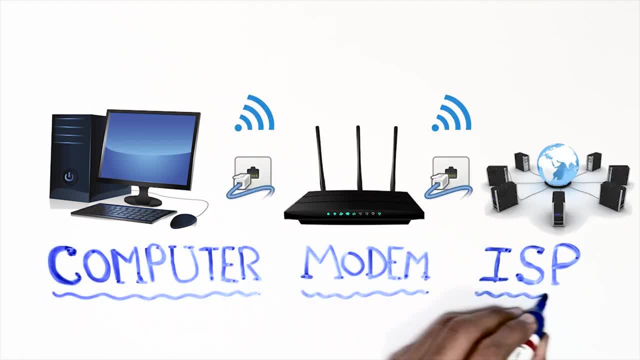 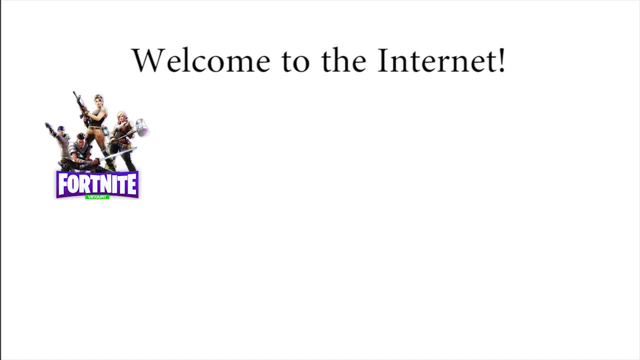 The modem then connects to an Internet Service Provider through a telephone line. Once you are connected to Internet, you can play games, listen to music or watch movie. send email messages, search for information, chat online, buy and sell products. do online banking. 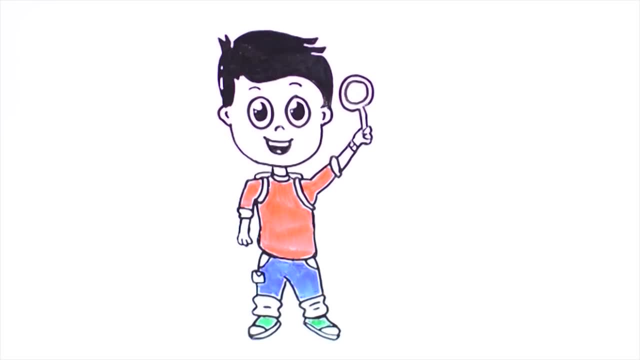 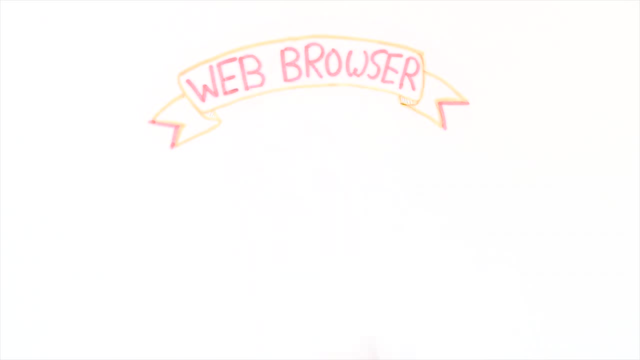 Once I am connected to the Internet, how will I view the information? For that, you will use a web browser installed on your device. A web browser is a software which is used to connect to the Internet. For that, you will use a web browser installed on your device. 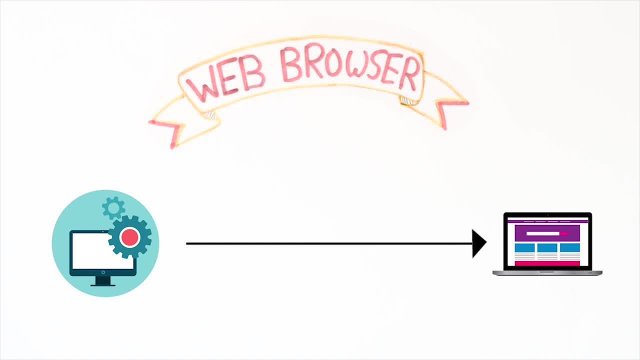 A web browser is a software which is used to connect to the Internet. A web browser is a software which is used to connect to the Internet. A web browser is a software which is used to connect to the Internet, For example, Google Chrome, Internet Explorer, Firefox, Safari, etc. 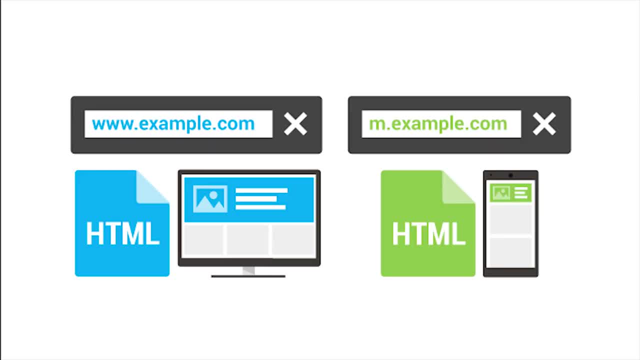 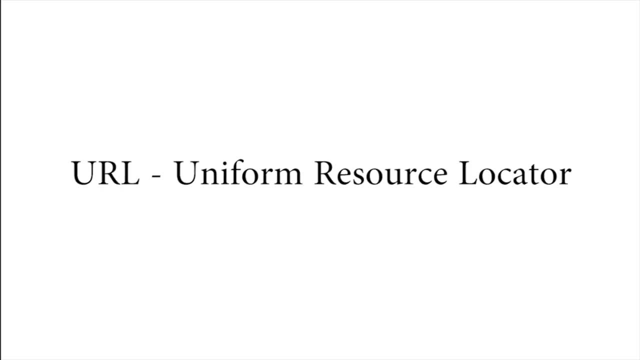 In the web browser you can directly type the URL of the website you wish to view. The URL is a short form for a Uniform Resource Locator. It is the address of a website or web page. For example, to go to SOF Olympia Trainer site. 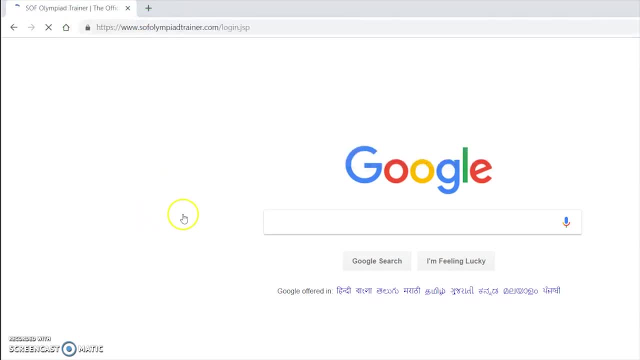 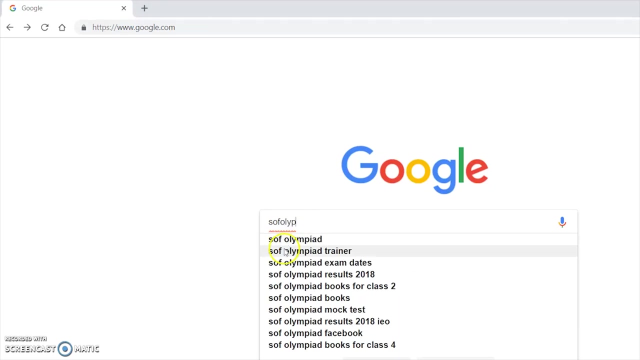 you will type wwwsofolympiatrainercom. You need to know the URL of the website you wish to visit. If you do not know the URL, you can use the search engine to look for the information. For example, you can search for SOF Olympia Trainer in the search engine.